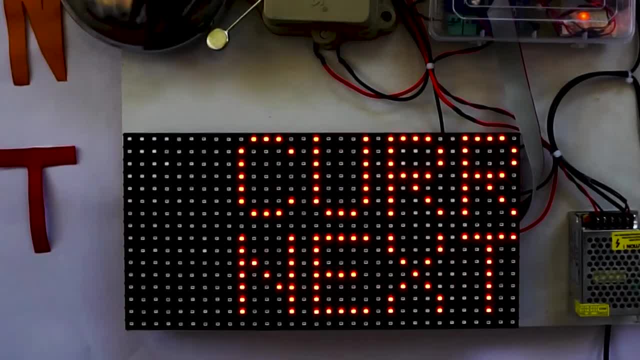 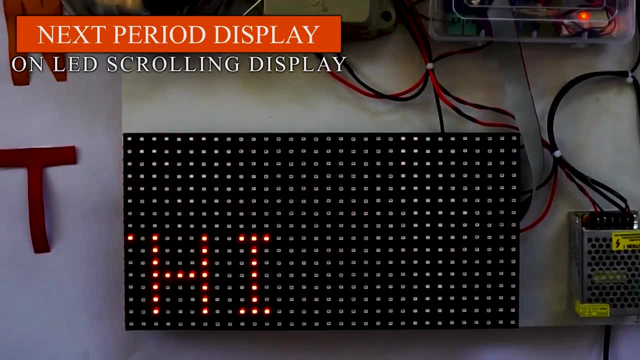 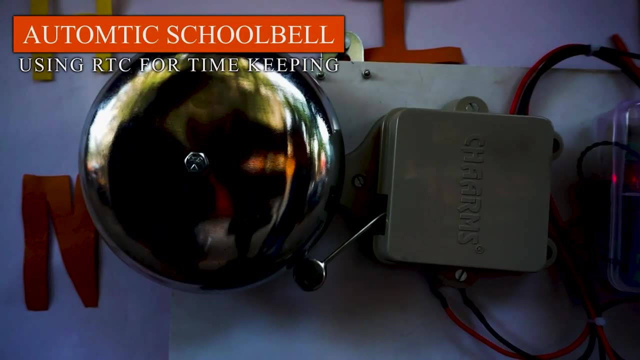 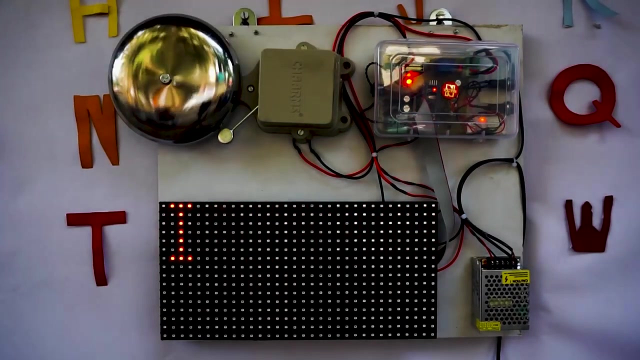 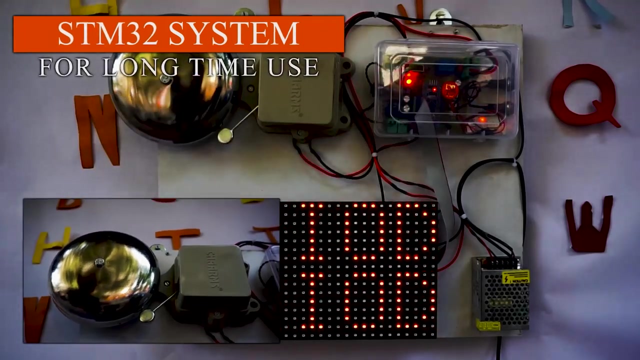 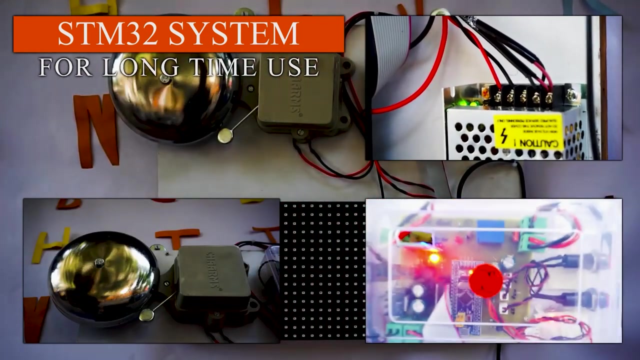 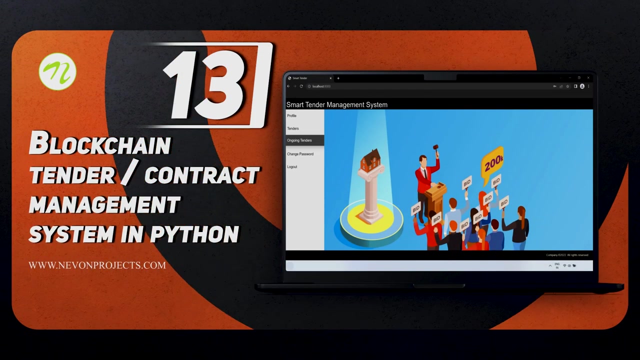 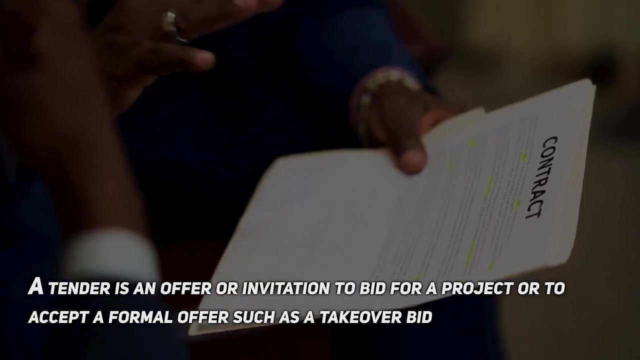 increased for more efficiency. increased efficiency, apprehensive waste, negative itself. good сторон ヽ ノ シี้ news, news, news, news, news, news news. A tender is an offer or invitation to bid for a project or to accept a formal offer, such as a takeover bid. 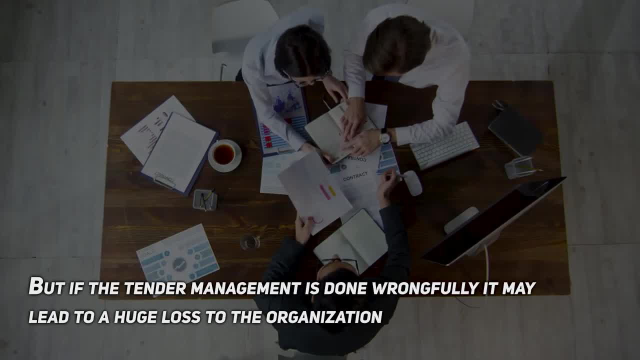 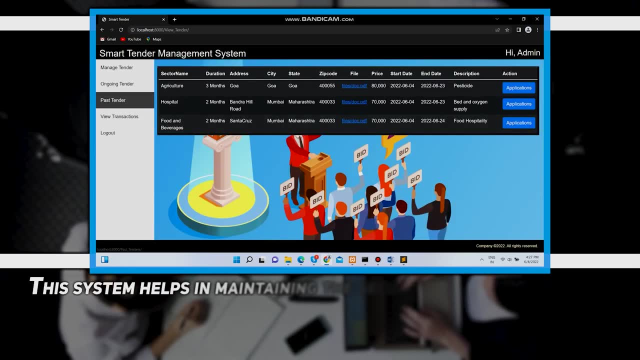 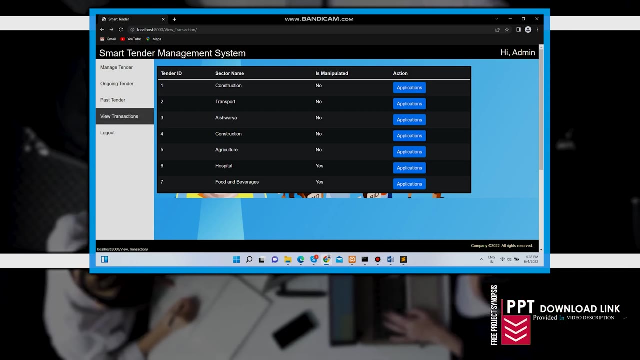 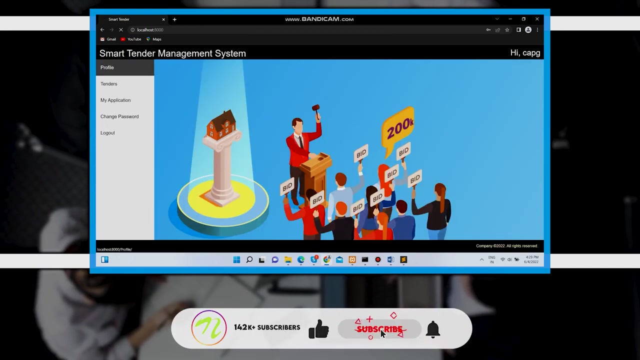 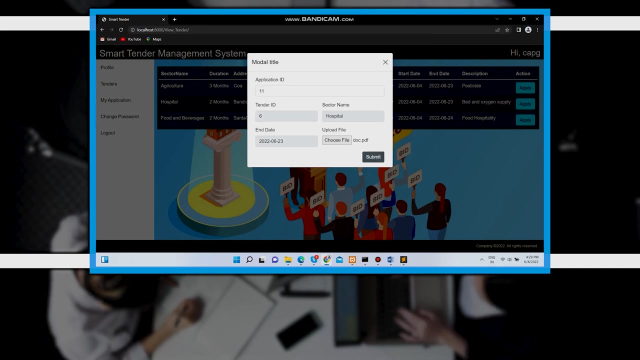 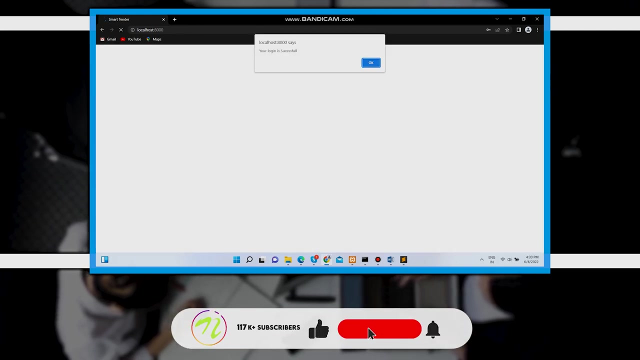 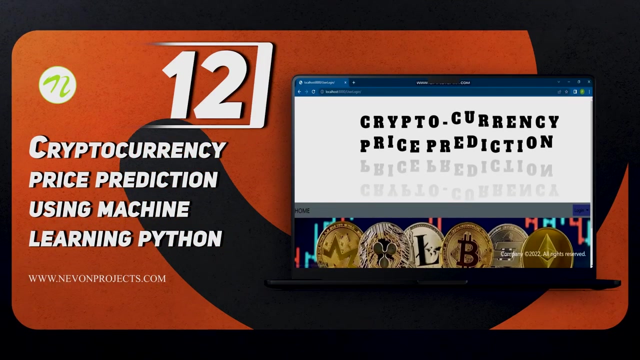 But if the tender management is done wrongfully, it may lead to huge loss through the organization. Let us check out this blockchain-based tender contract management system. This system helps in maintaining the security and efficiency of each tender. Cryptocurrency price prediction using machine learning- Python. 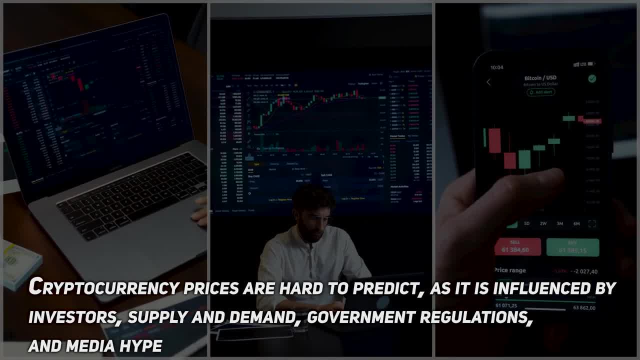 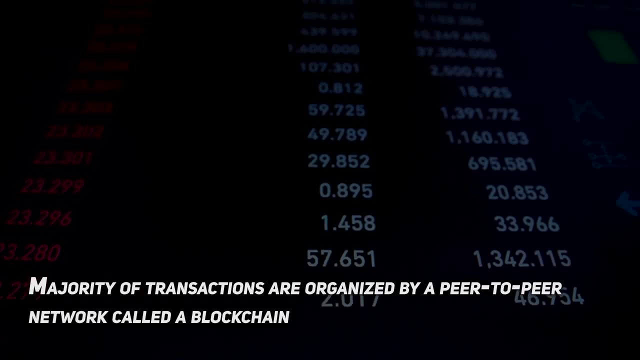 Cryptocurrency prices are hard to predict as it is influenced by investors, supply and demand, government regulations and media hype. Majority of transactions are overpriced, organized by a peer-to-peer network called a blockchain. Let us check out this cryptocurrency price prediction system. 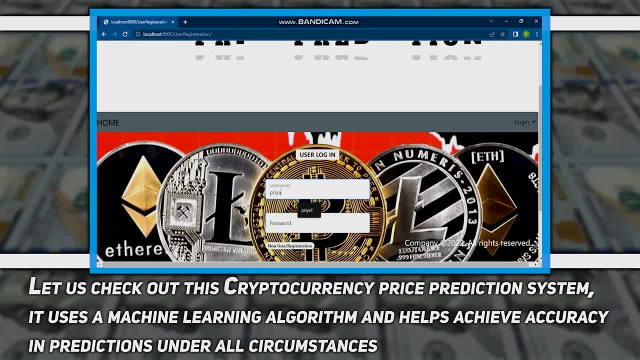 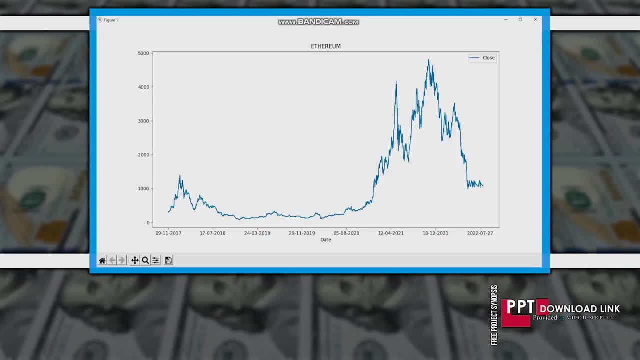 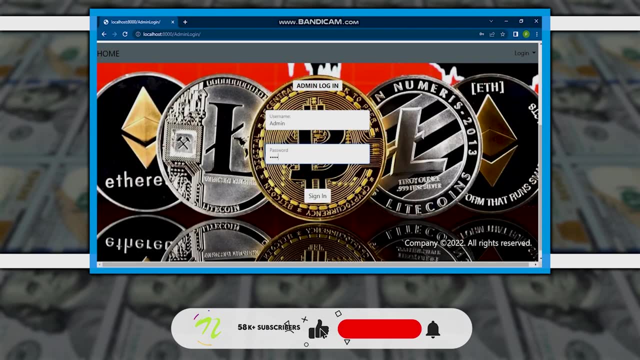 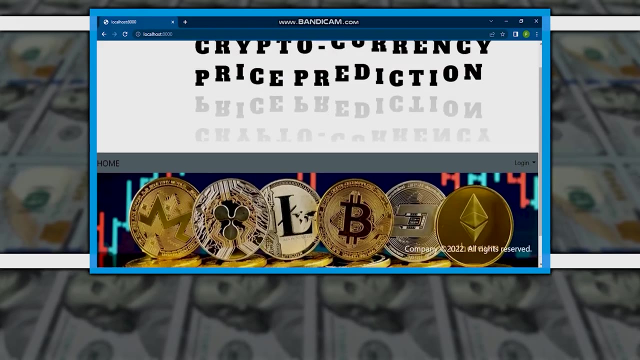 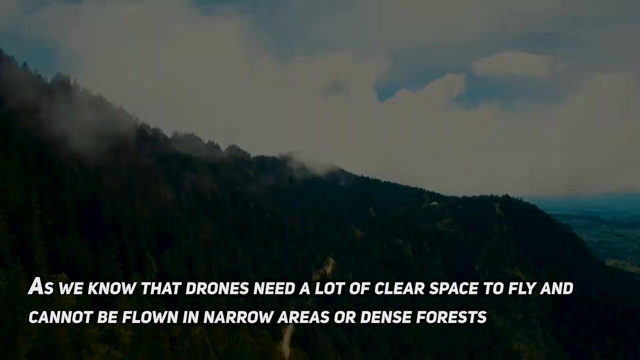 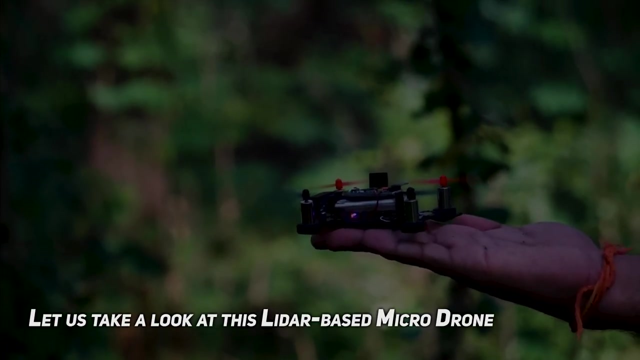 It uses a machine learning algorithm and helps achieve accuracy in predictions under all circumstances. As we know that drones need a lot of clear space to fly and cannot be flown in narrow areas or dense forests, Let us take a look at this Lidar-based micro drone. 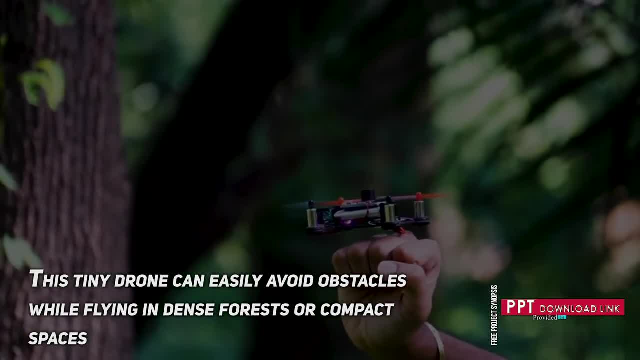 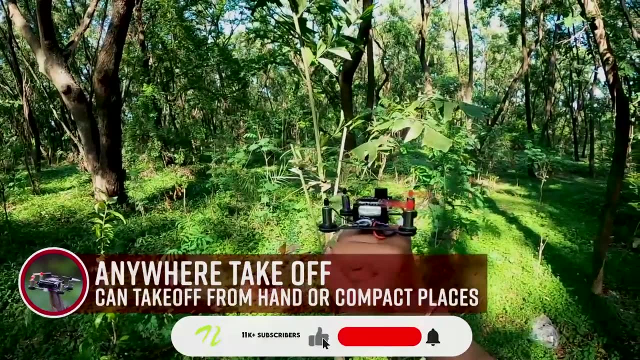 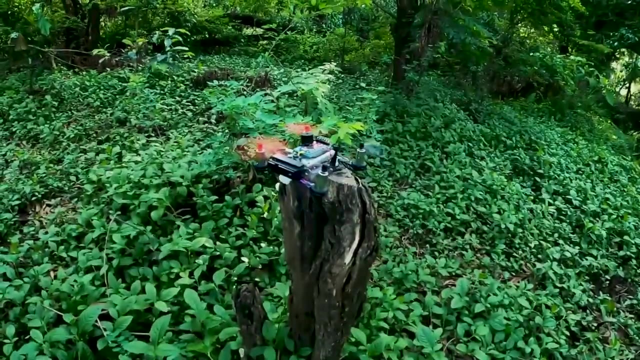 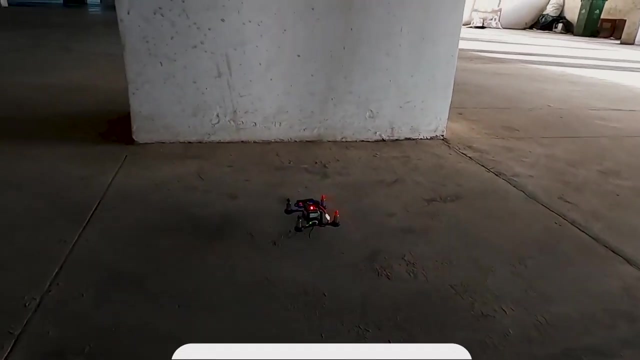 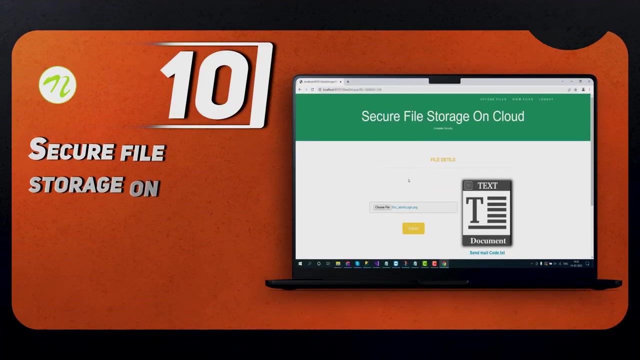 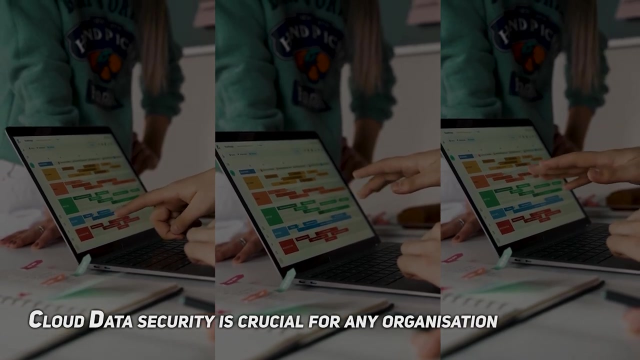 This tiny drone can easily avoid obstacles while flying in dense forests or compact spaces. Let us take a look at this Lidar-based micro drone. Secure file storage on cloud using hybrid cryptography. Cloud data security is crucial for any organization. It is necessary to give or revoke access. 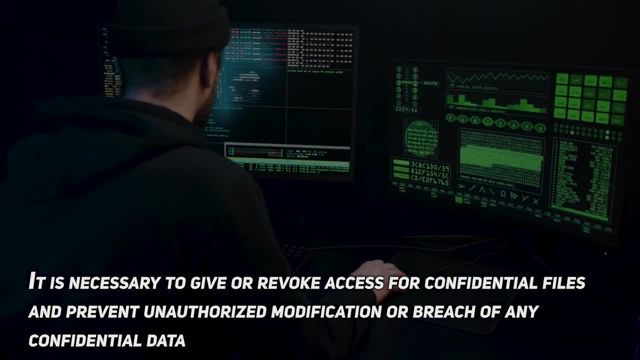 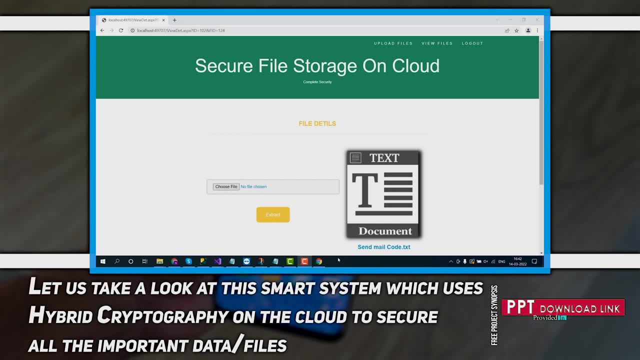 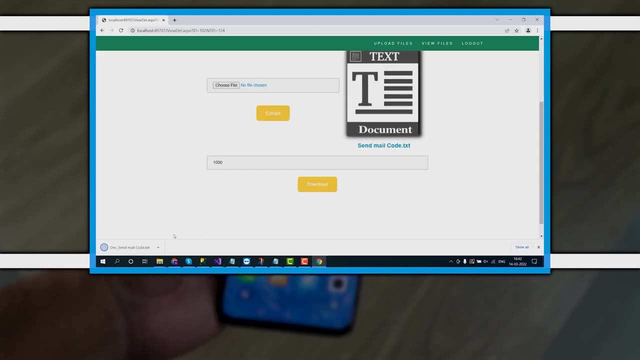 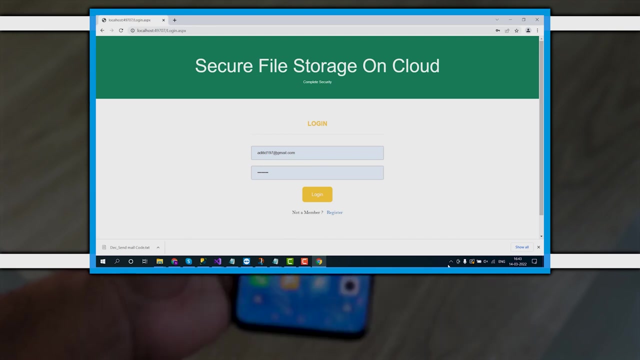 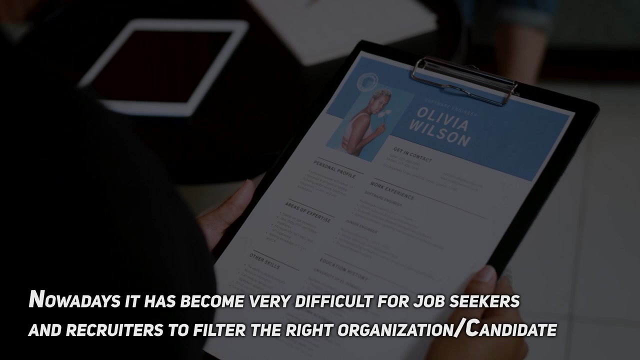 for confidential files and prevent unauthorized modification or breach of any confidential data. Let us take a look at this smart system which uses hybrid cryptography on the cloud to secure all the important data or files: Android job portal system app. Nowadays, it has become very difficult for job seekers and recruiters 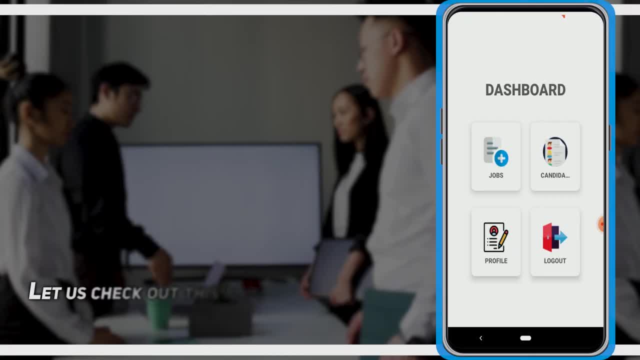 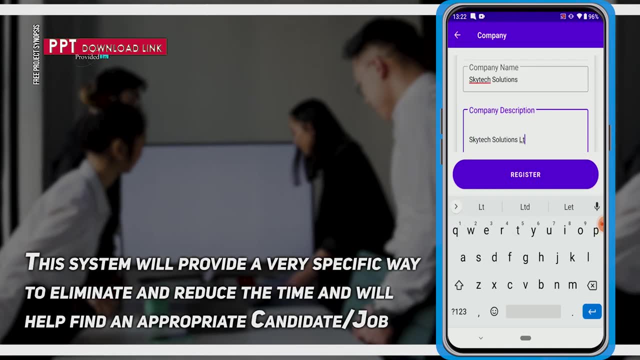 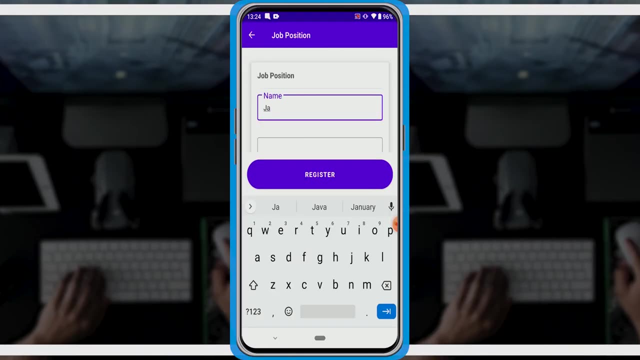 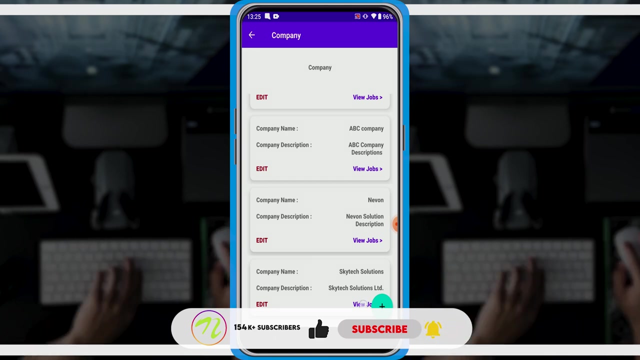 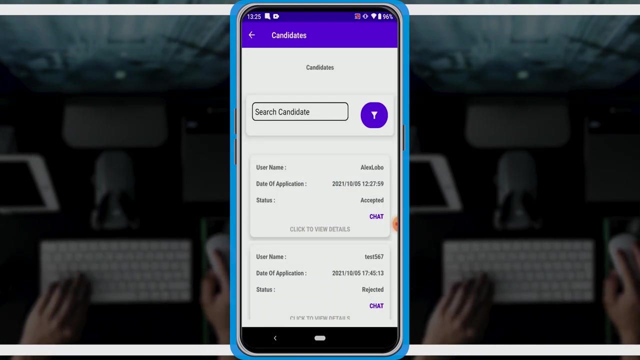 to filter the right organization or candidate, Let us check out this Android-based job portal system. This system will provide a very specific way to eliminate and reduce the time and will help find an appropriate candidate or job. It is a very simple and easy way to filter all the data. 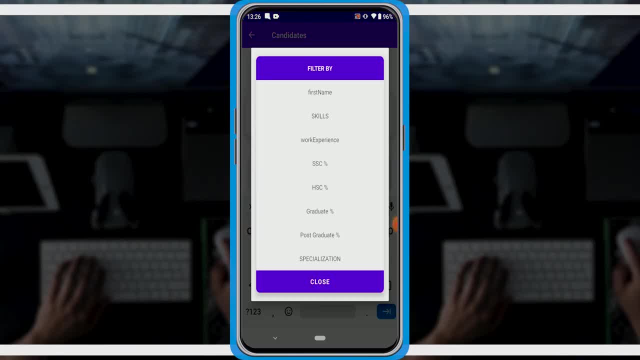 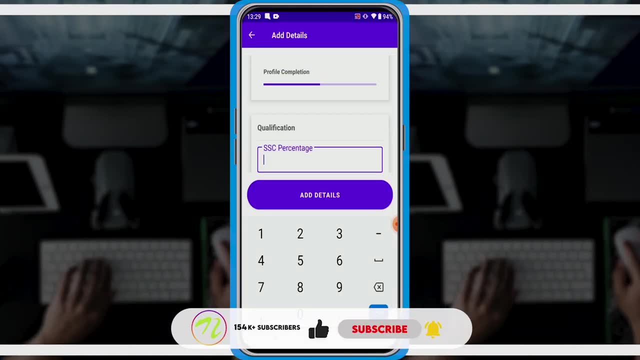 At the same time, it can be useful for the job to create a list of the time and hours of the job that was posted or the time that was left. The job identity of job is hidden at the top, But the job identity of the job is visible and automatic. 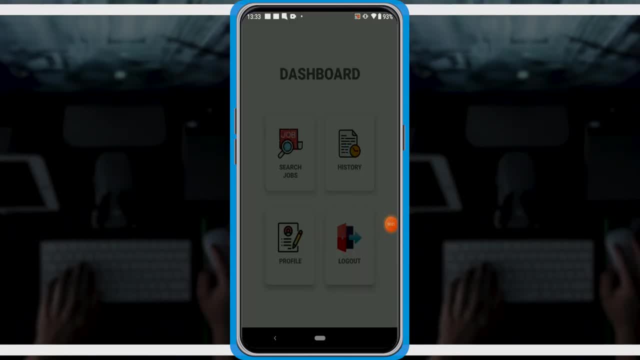 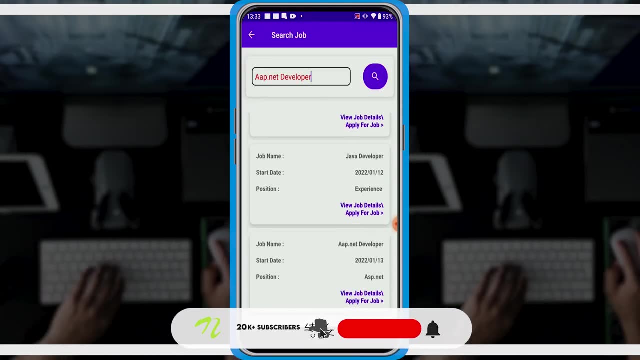 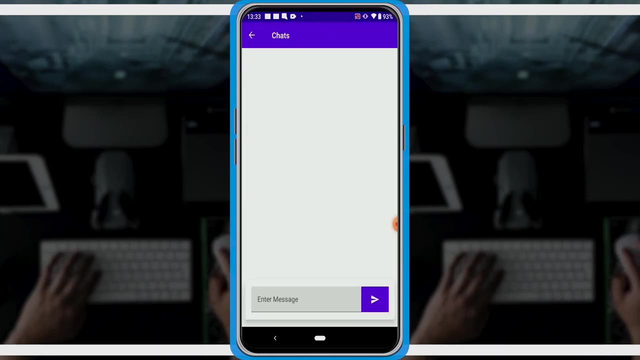 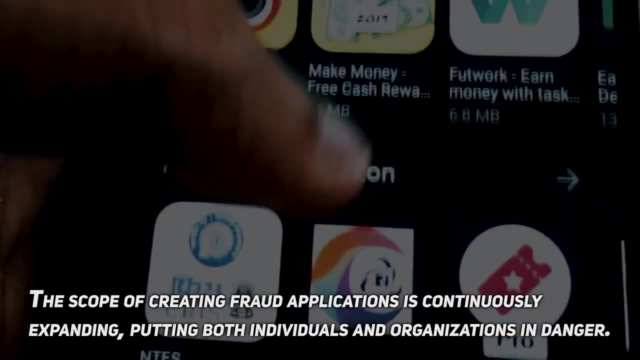 If you want to, using the job ID, you can attach the job ID on your tablet or tablet with your smartphone. You can use this method at home. Detecting Fraud Apps Using Sentiment Analysis. The scope of creating fraud applications is continuously expanding, putting both individuals. 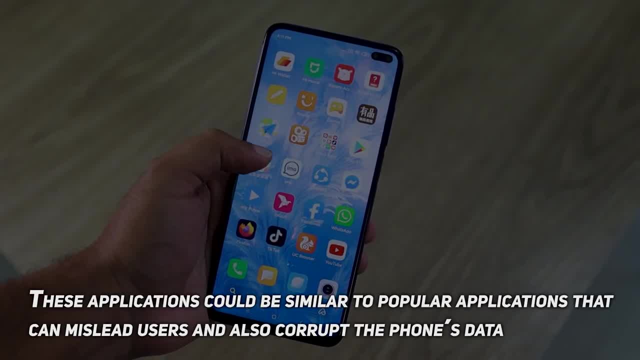 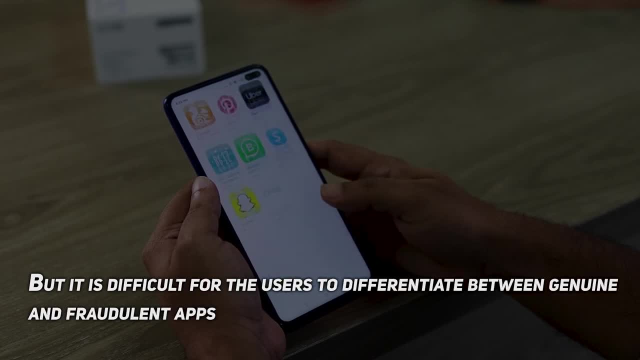 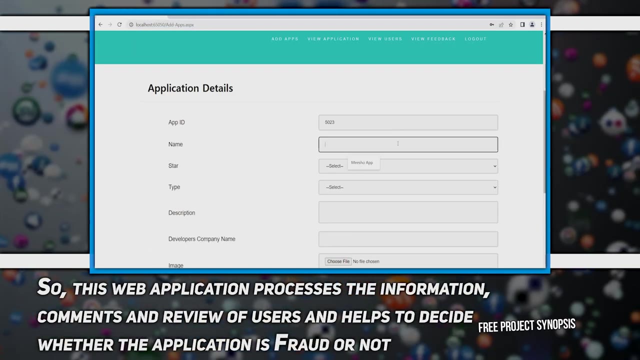 and organizations in danger. These applications could be similar to popular applications that can mislead users and also corrupt the phone's data, but it is difficult for the users to differentiate between genuine and fraudulent apps. So this web application processes the information, comments and reviews of users and helps to 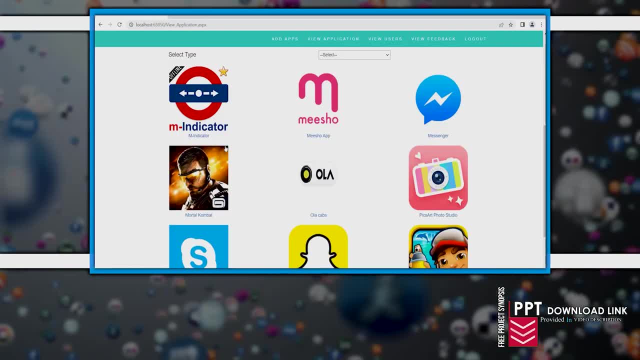 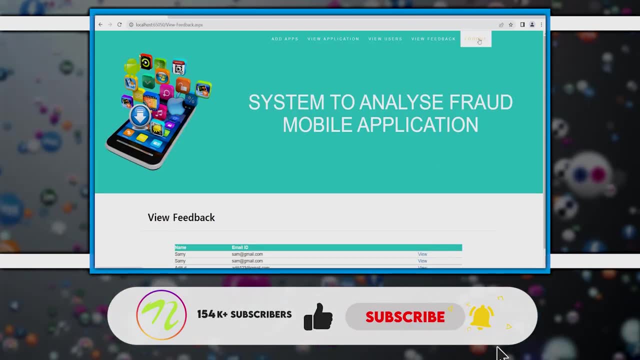 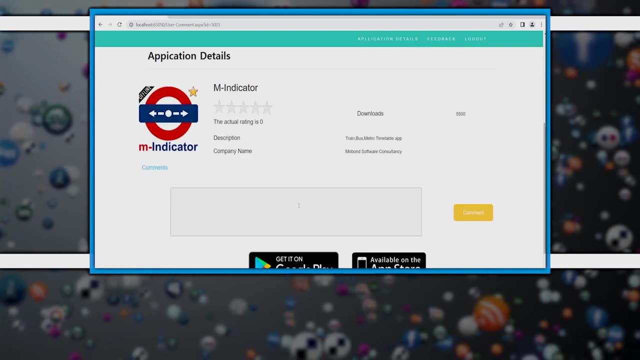 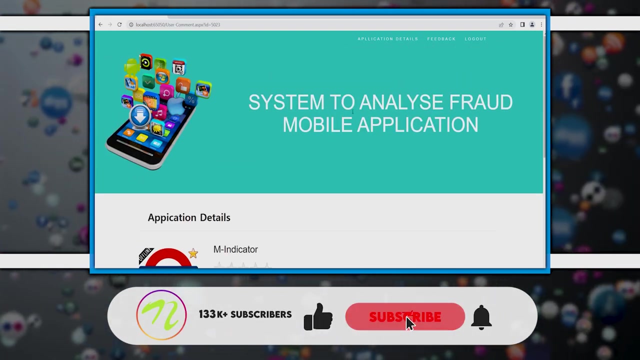 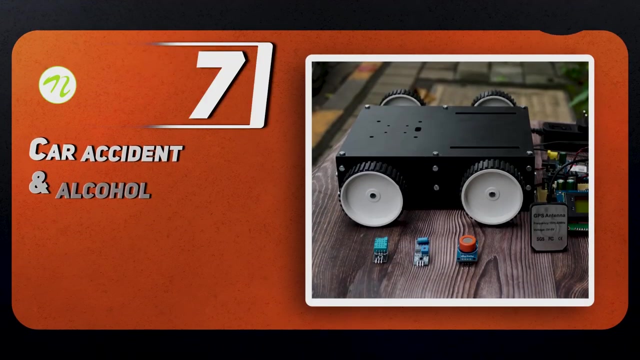 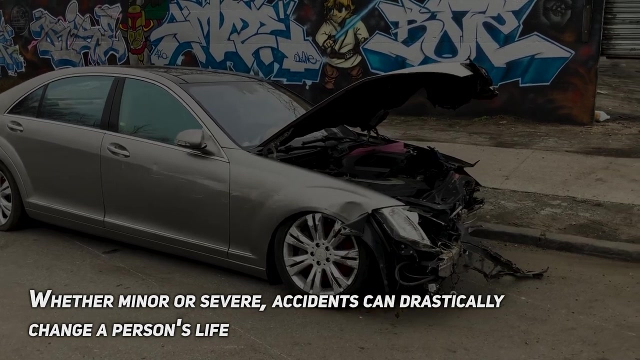 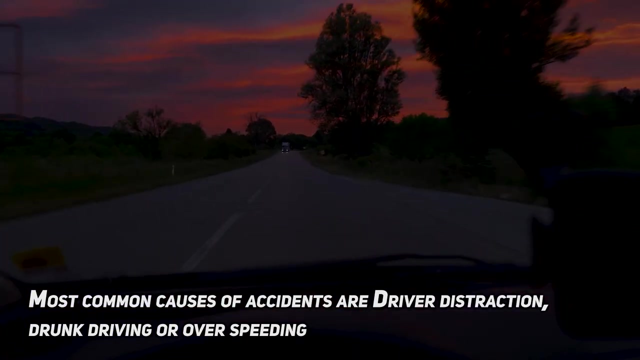 decide whether the application is fraud or not. Car accidents, alcohol detector and recorder blackboards, Whether minor or severe accidents can drastically change a person's life. Most common causes of accidents are driver distraction, drunk driving or over-speeding. Things that you should be careful about while dealing with accidents are: 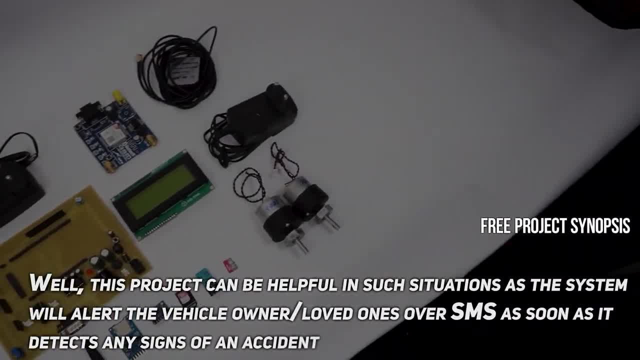 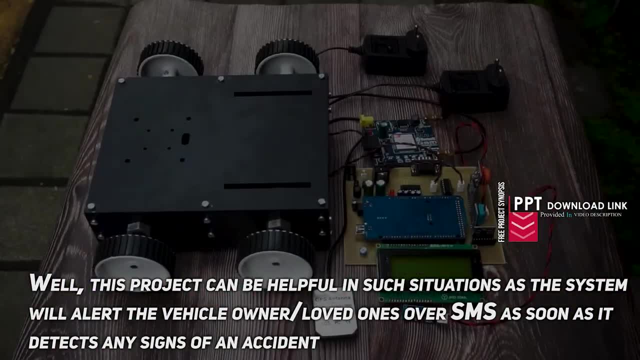 1. Self-indulgence. 2. Well, this project can be helpful in such situations, as this system will alert the vehicle owner or their loved ones over SMS as soon as it detects any signs of an accident. So this is the wireless car black box system, which is powered by Ardion Omega. 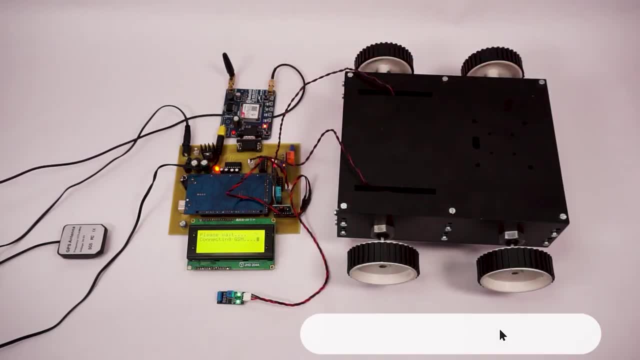 So now let's turn on the GSM modem so that we can configure our number and once that is done so, whenever anything happens, the SMS will be sent on this particular registered number. So, as you can see, we got an SMS saying that this number has been configured. 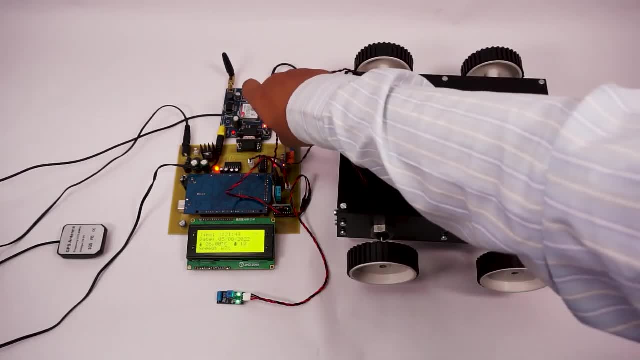 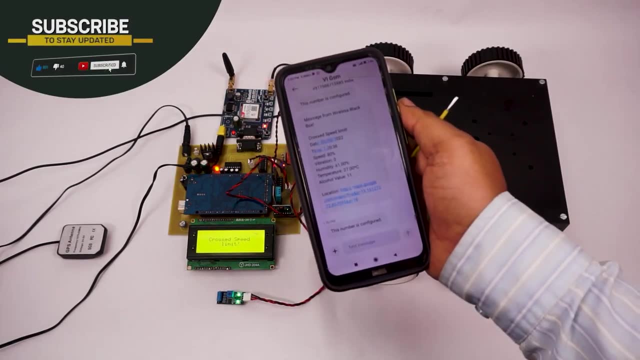 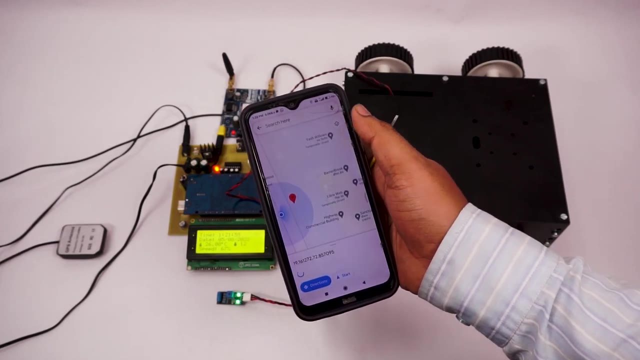 So now we will adjust the motor speed using a trim pot to simulate high speed of the car. So, as you can see, it is saying that the speed limit has been crossed, And we also got an SMS with GPS location of the vehicle where it crossed the speed limit. 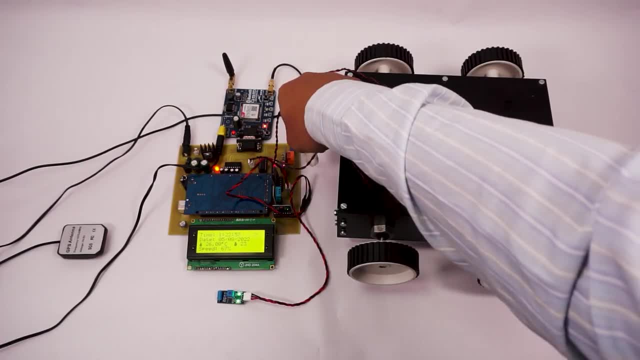 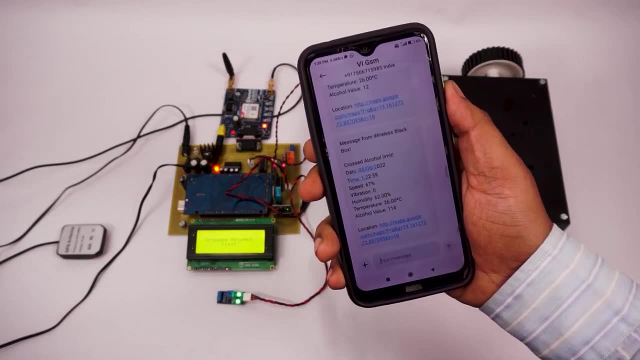 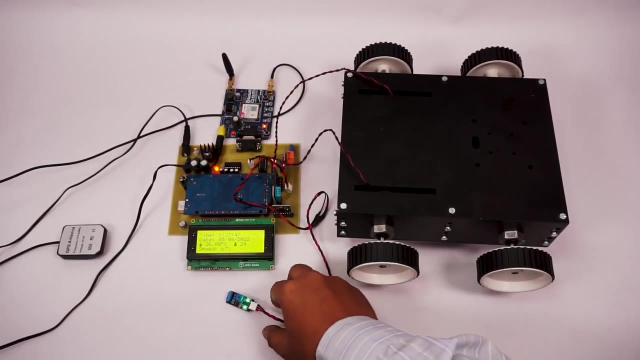 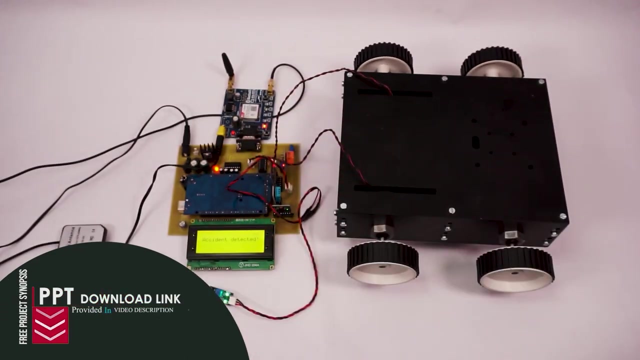 So now let's simulate alcohol. Suppose alcohol was detected In the vehicle and we got another SMS message about the event, along with the GPS coordinate. Now we will simulate vibration or accident. So whenever an accident happens, high levels of vibration will be detected. 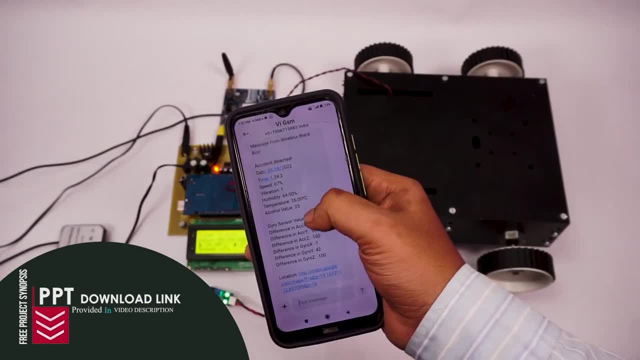 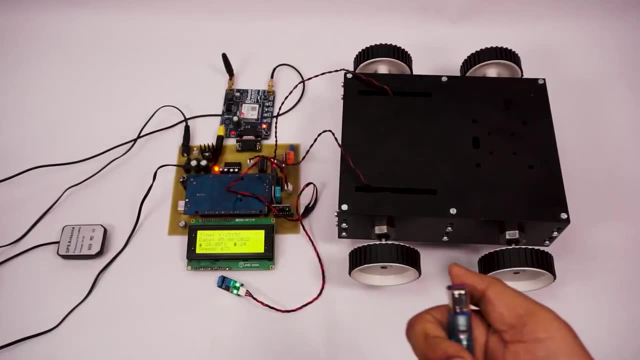 So now, as soon as the vibration or accident is detected, we got the values of the sensor as well as the GPS coordinate where the accident was detected. Okay, So next we will simulate fire. Suppose the car caught fire or there was a fire incident. 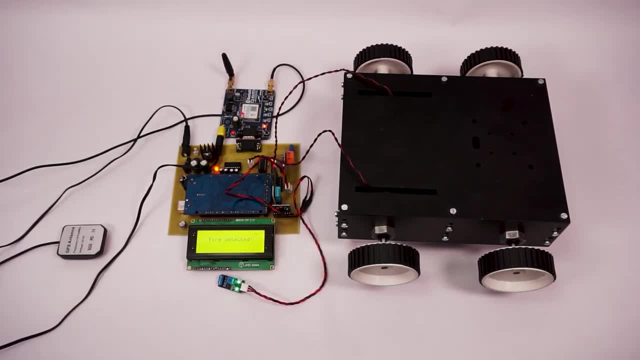 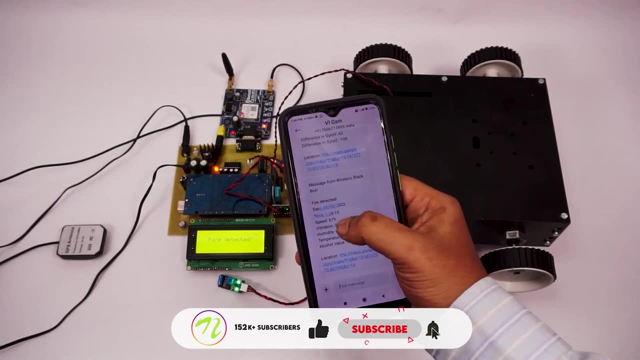 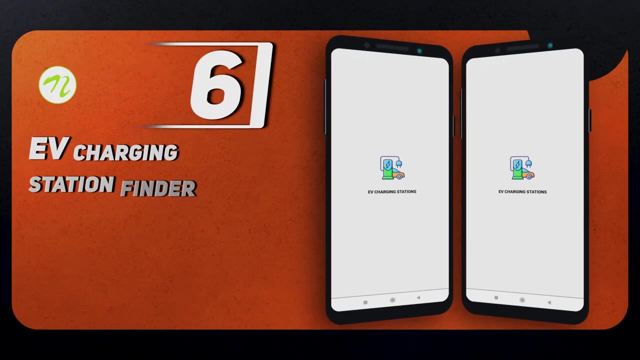 So now, in this case again, we are going to get a fire alert notification through SMS, along with the GPS coordinates of where it was detected. So this is the wireless car black box system, which is powered by Arduino, Mega EV Charging Station Finder and Slot Booking. Electric vehicles still fall short when it. 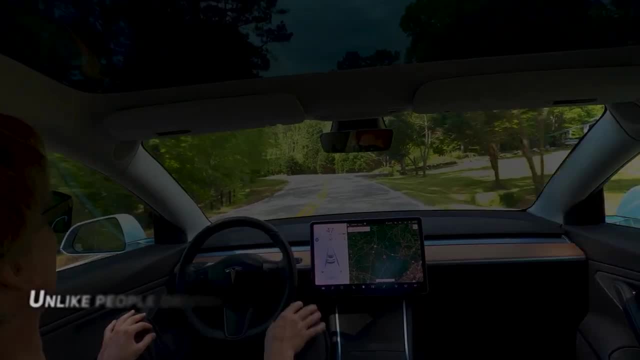 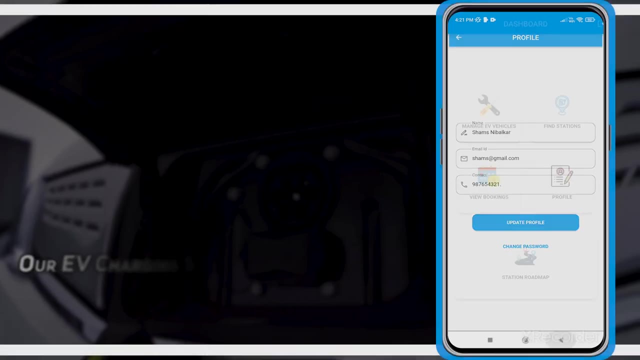 comes to Aspen. We are going to show you a few aspects, such as finding charging stations. Unlike people driving conventional cars, EV owners can't have their vehicles refueled at any fuel station. Our EV Charging Station Finder system has been developed to help EV drivers locate available. 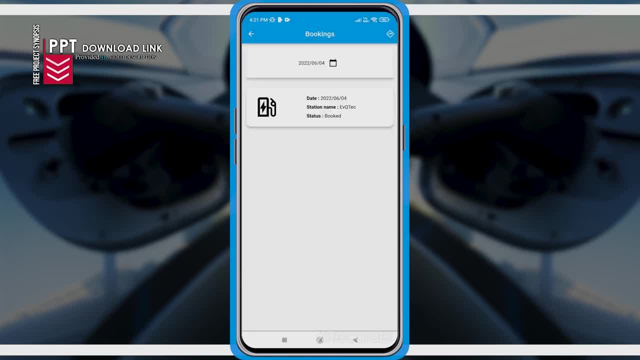 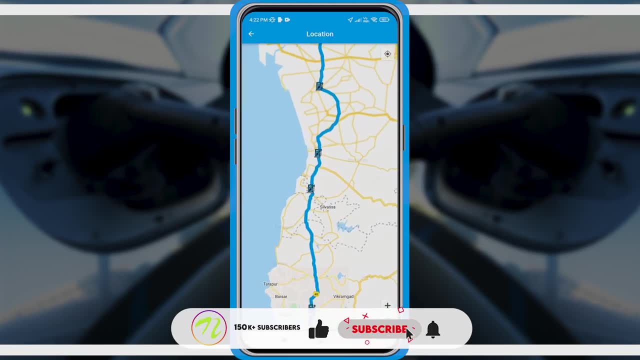 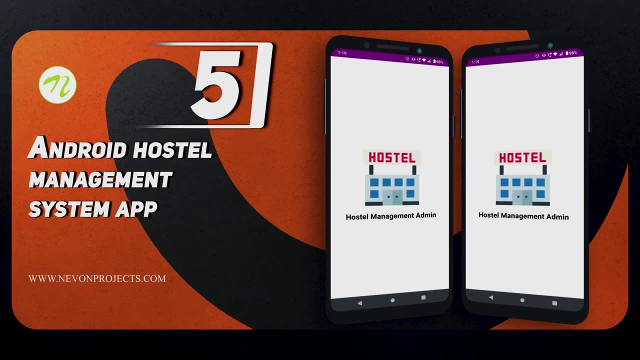 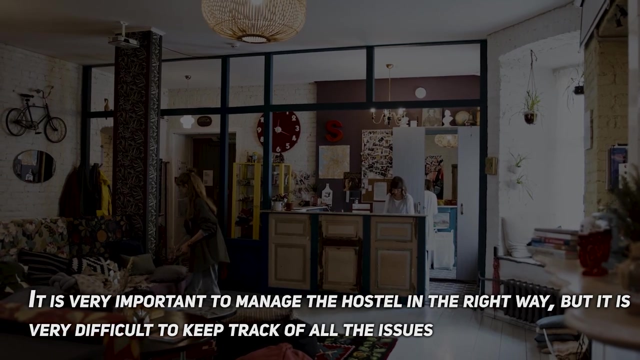 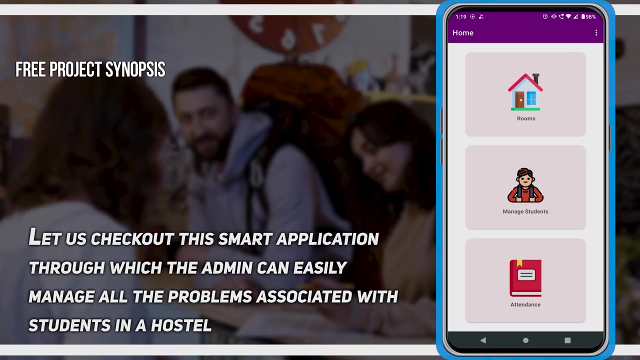 charging stations near them. The service is a little more expensive than the one in the A1 version, but we will show you how that works, So let's see how it works. Android Hostel Management System App. For a lot of inhabitants, a hostel is a home. 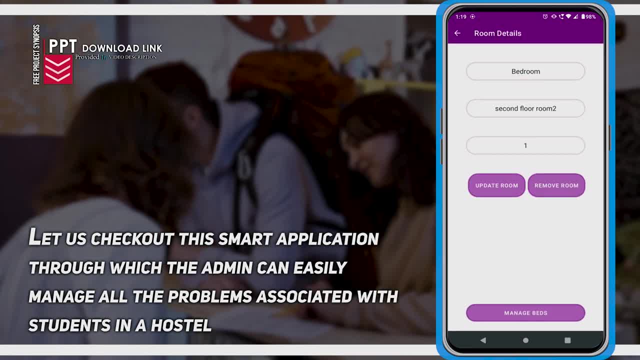 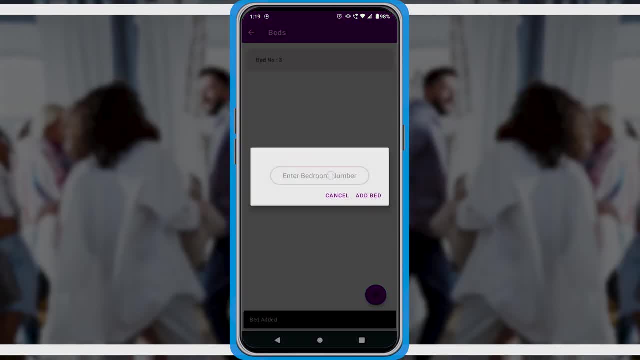 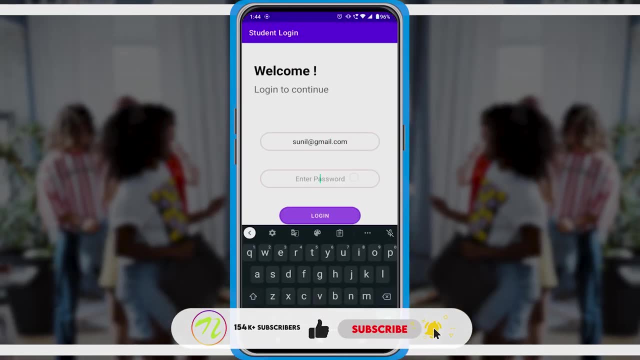 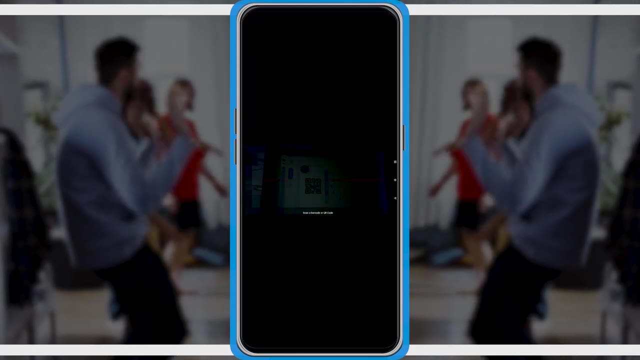 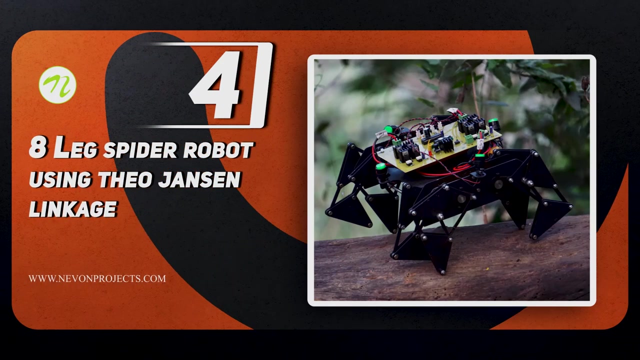 away from home. It is very important to manage the hostel in the right way, but it is very difficult to keep track of all the issues. Let us check out this smart application through which the admin can easily manage all the 8-Lake Spider Robot using Theo Jansen linkage. 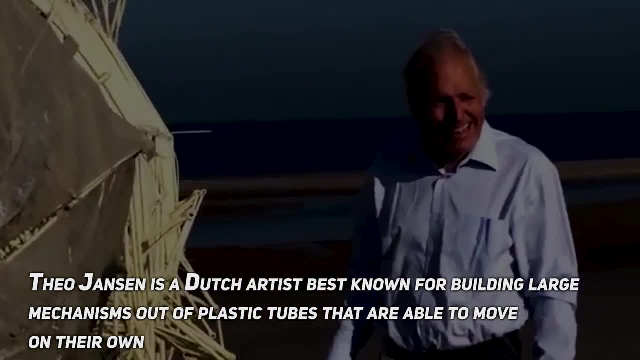 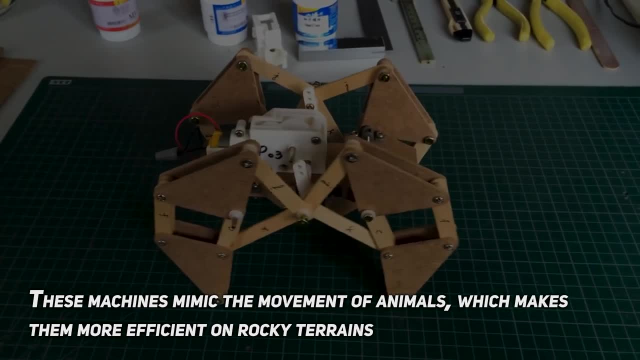 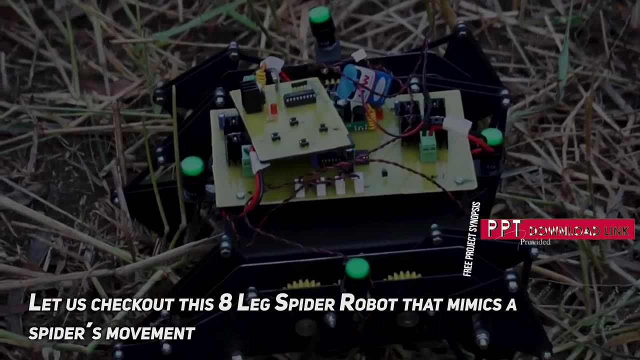 Theo Jansen is a Dutch artist best known for building large mechanisms out of plastic tubes that are able to move on their own. These machines mimic the movements of animals, which makes them more efficient on rocky terrains. Let us check out this 8-Lake Spider Robot that mimics a spider's movement. 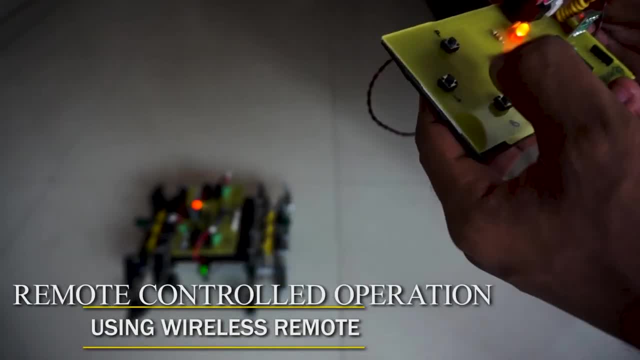 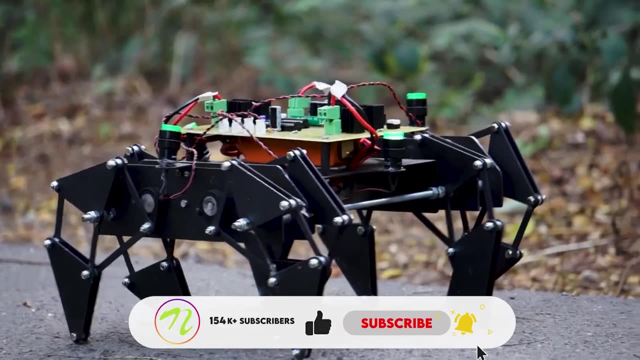 Let us see, how cool it is: 1. Crowding, 3. Cracking, 4. Knocking, 5. Scießing, 6. Cracking, 7. Cracking, 8. Crack, 9. Cracking, 10.. 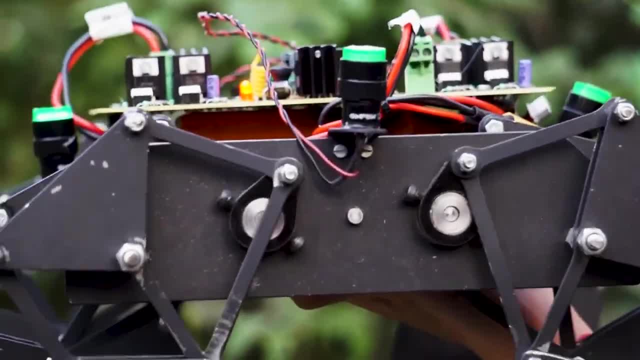 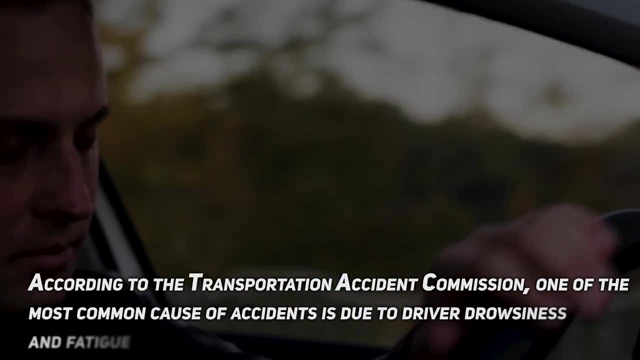 Cracking, 11. Cracking, 12. Cracking, 12. Cracking, 13.. Driver Drowsiness Detection System using Python. According to the Transportation Accident Commission, one of the most common cause of accidents is due to driver drowsiness. 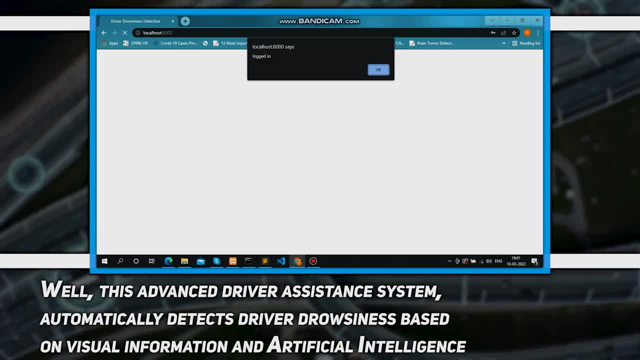 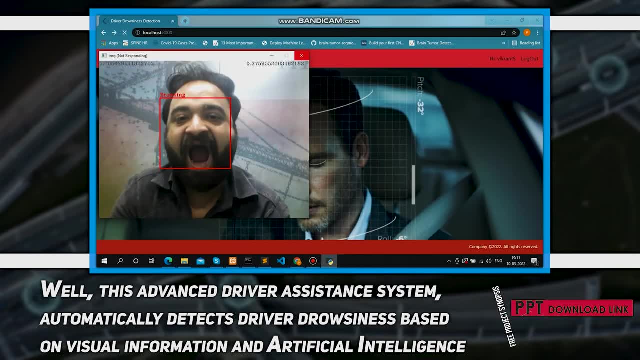 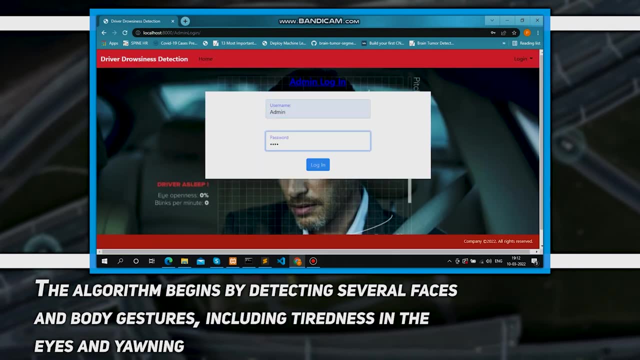 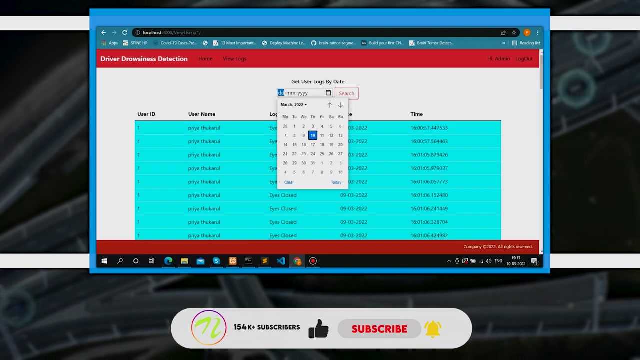 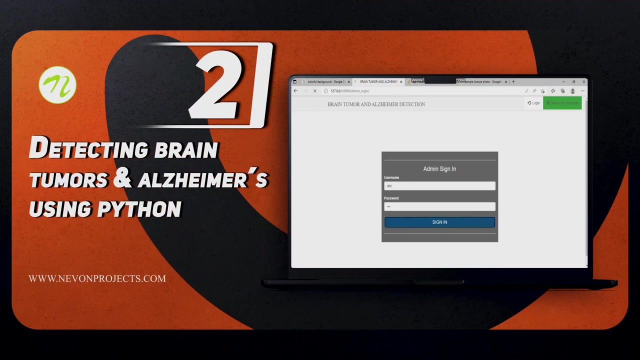 and fatigue. Well, this advanced driver assistance system automatically detects driver drowsiness, based on visual information and artificial intelligence. The algorithm begins by detecting several faces and body gestures, including tiredness in the eyes and yawning, Detecting Brain Tumors and Alzheimer's Using Python. 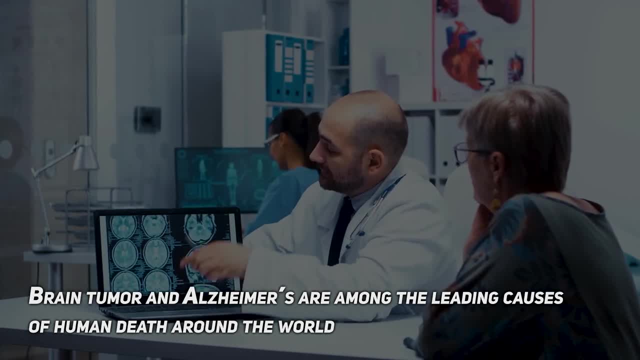 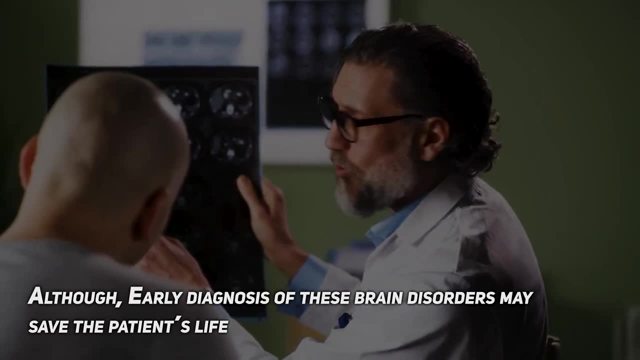 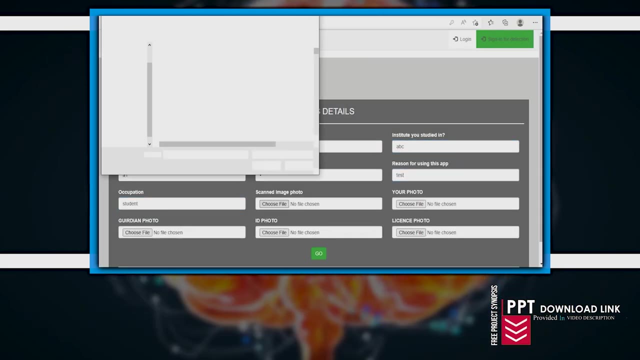 Brain tumor and Alzheimer's are among the leading causes of human death around the world. Although polydiagnosis of these brain disorders may save the patient's life, Here we have an intelligent system for detecting brain disorders at an early stage. Where are the traces of brain tumors found? 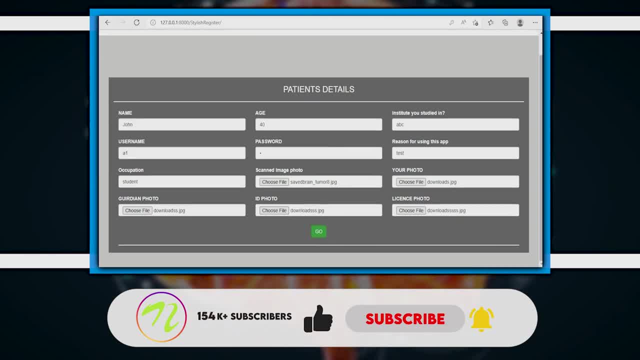 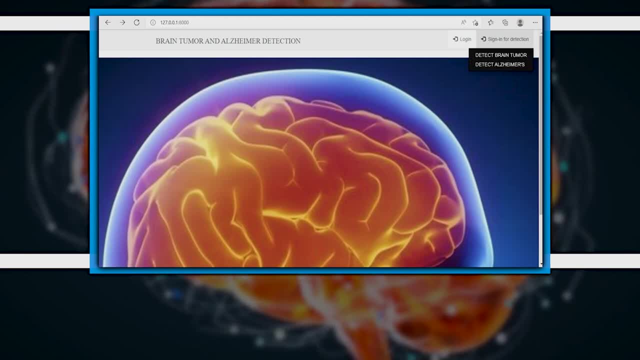 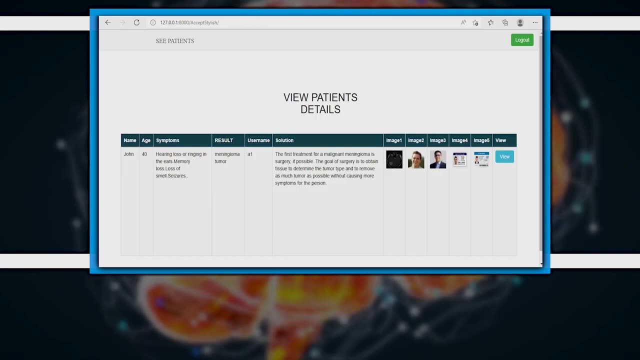 A- In the brain and in the body. B- In the brain and in the body. C- In the body and in the body. Can brain tumors be detected in the body? A- In the body and in the body? 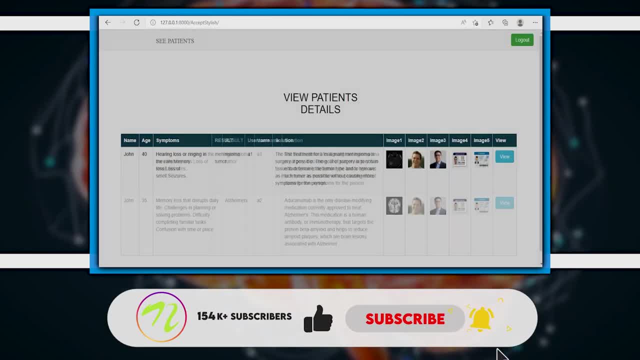 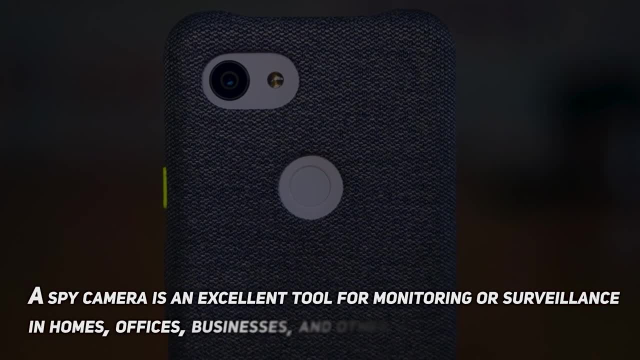 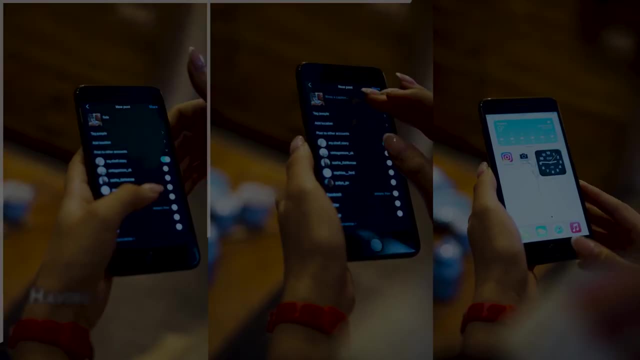 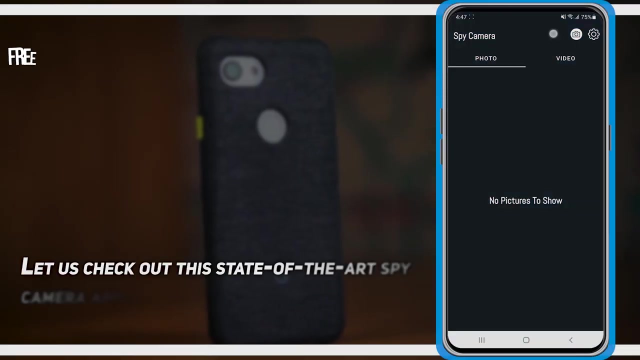 Spy Camera Android App. Spy Camera is an excellent tool for monitoring or surveillance in homes, offices, businesses and other work environments. Having a spy camera handy can also help to absorb and record the activities, which you can review later. Let us check out this state of art spy camera application that can help you capture anything.